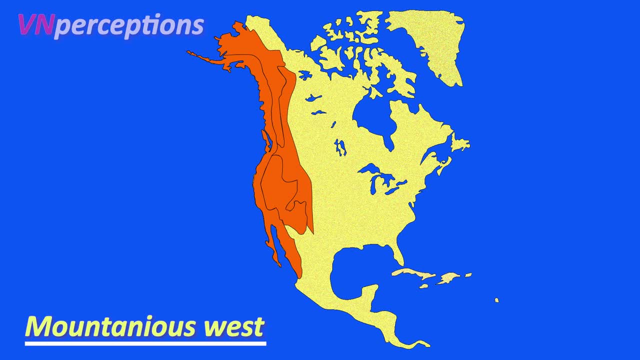 called Cordilleras. When I say Cordilleras, they refer to an extensive chain of mountains or mountain ranges, and the Cordilleras extend from Canada all the way to the isthmus of Panama Broadly. this region can be classified as the Rocky Mountains, the Inter-Mountain Basin. 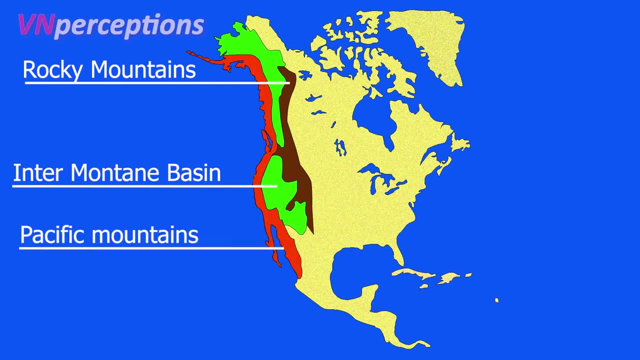 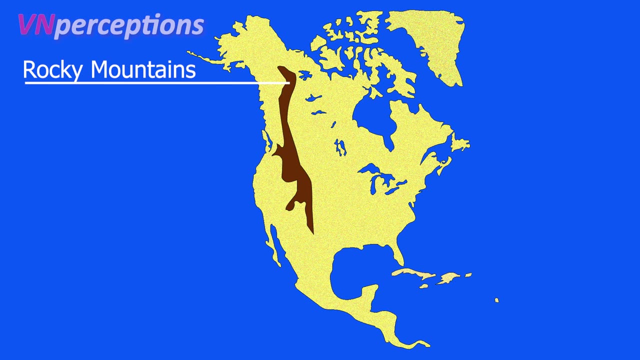 and the Plateaus. 3. When I talk about the Rocky Mountains, they are part of a system of parallel mountain ranges known as Cordilleras, and these Rocky Mountains stretch some 4830 km from the province of British Columbia to the US state of New Mexico. 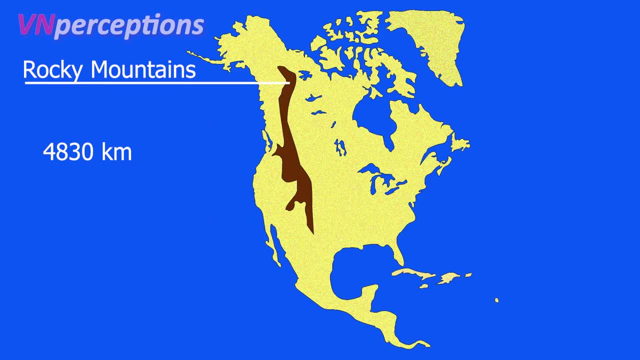 4. The Rockies are distinct from the Pacific Coast Ranges, the Cascade Range and the Sierra Nevada, which all lie further to the west, and the Rockies are distinct from the Pacific Coast Ranges. Well, the Rocky Mountains include at least 100 separate ranges, which are generally divided. 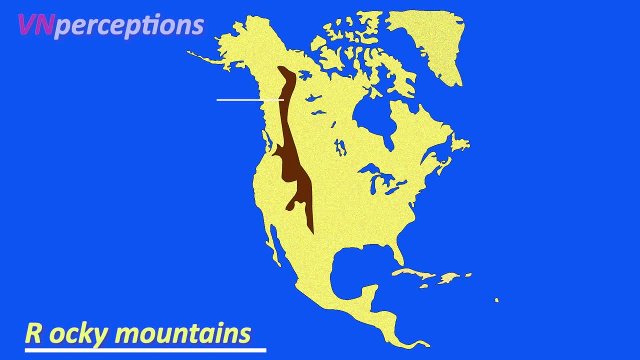 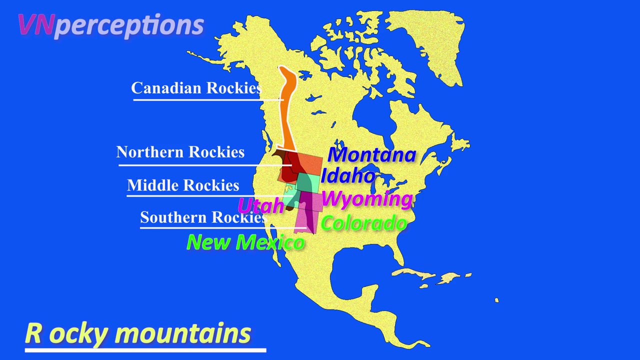 into four broad groups, And they are: the Canadian Rockies, the Northern Rockies of Montana and Northeastern Idaho, the Middle Rockies of Wyoming, Utah and Southeastern Idaho, the Southern Rockies mainly in Colorado and New Mexico. Well, these four subdivisions differ from each other in terms of geology, ie origin. 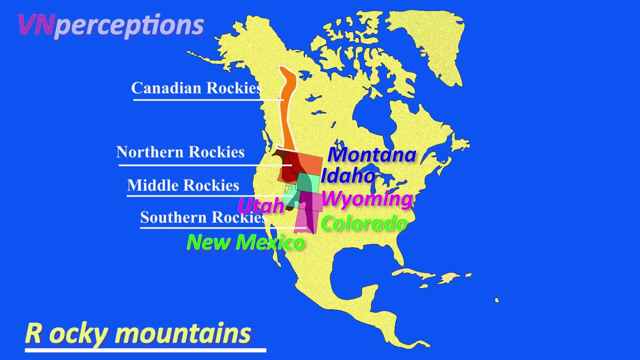 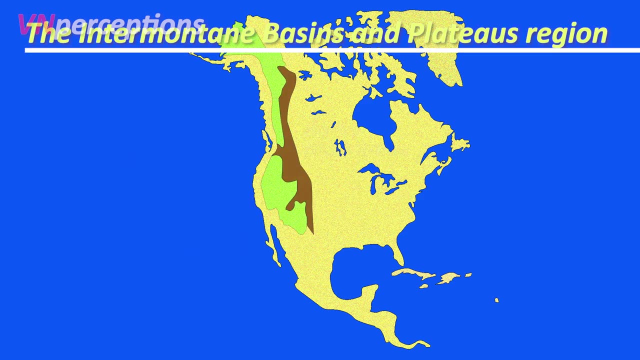 age, and even the type of rocks and physiography, landforms, drainage, soil, and yet they share the physical attributes of high elevation. 5. Now we come to the Intermontane Basins and Plateau Regions. This is flanked on the west by the major Pacific Coastal Mountain Ranges, and on the east we 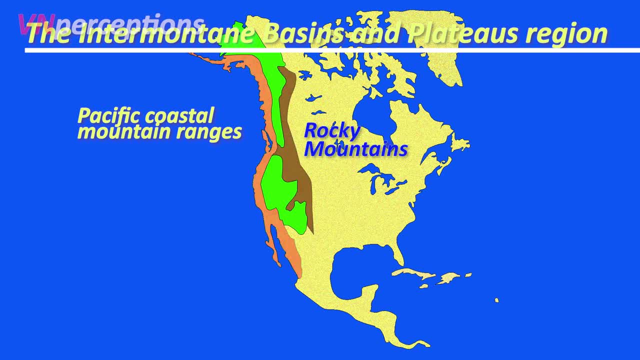 know it is Rocky Mountains. 6. In broad terms, the region consists of three distinctive sub-regions, and that is the Colorado Plateau, the Columbia Plateau and the Southern Basins. 7. The Intermontane region is characterized by sparse population, concentrated in a few major 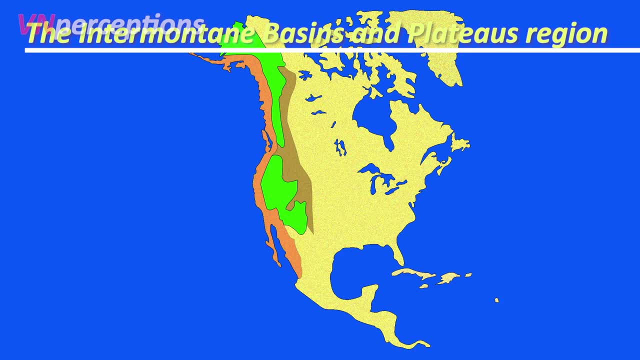 urban centers, a relatively isolated setting between extensive mountainous areas and very high serine descents. 8. The Intermontane region is densely populated with sunlight and has good water resources, such as fresh water and soft scrubbing. 9. 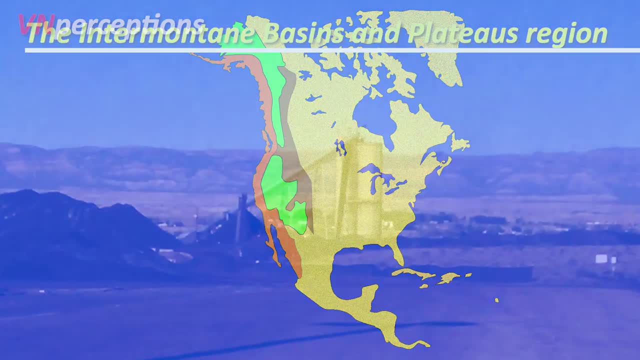 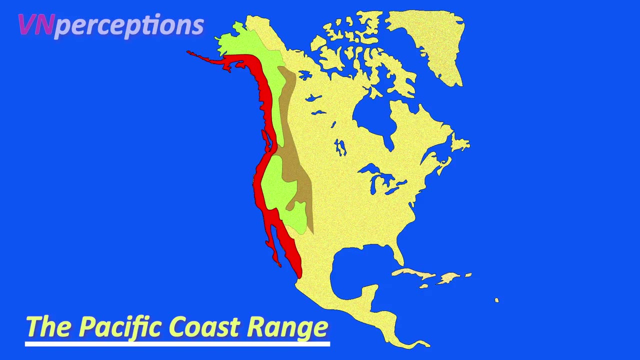 More bases and arid and semi-arid climate patterns, limited water assets and considerable mineral resources. 10. Coming to next, and that is the Pacific Coast Ranges. Now, these are the series of mountain ranges that stretch along the west coast of North. 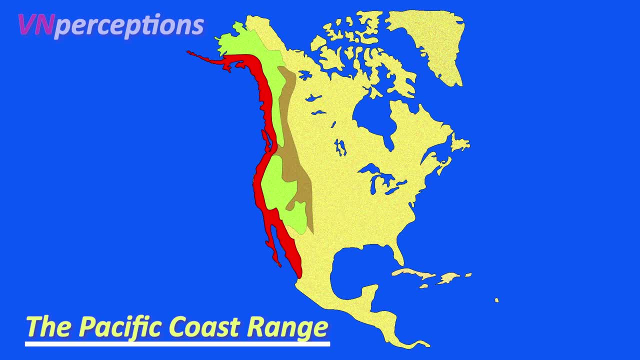 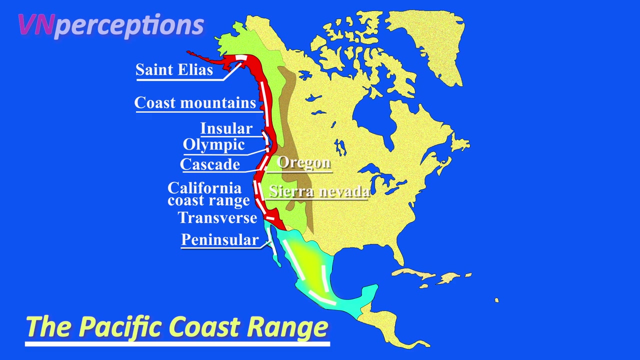 America from Alaska south to northern and central Mexico. Now it comprises of St Elias Mountains, Coast Mountains, Insular Mountains, Olympic Mountains, Cascade Range, Sierra Nevada, Oregon Coast Range, California Coast Ranges, Transverse Ranges, Peninsular Ranges and the Sierra Madre Mountain System of Mexico. 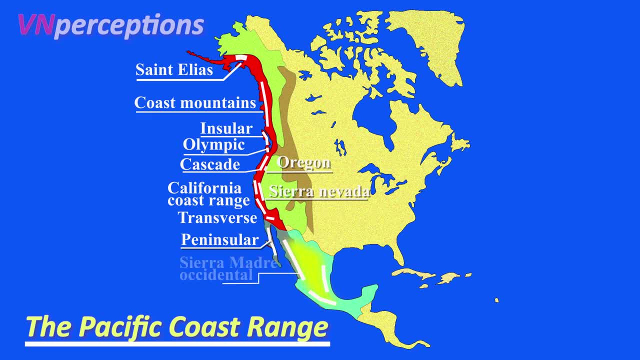 Now it consists of Sierra Madre Occidental, ie to the West, Sierra Madre Oriental, ie to the East, and Sierra Madre del Sur, to the South. These are the mountains. These ranges enclose the Great Central Mexican Plateau, which itself is a part of the system, although the northern portion of the plateau also is considered to be the basin and a range province in the United States. 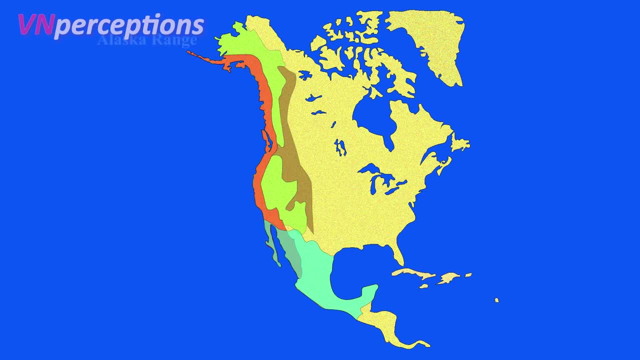 Then we left out one more range, which is a part of the American Cordillera, ie Alaska Range. This range is the highest in the world outside Asia and Andes. It stretches over 6.5 km, Like a crescent moon across central Alaska. 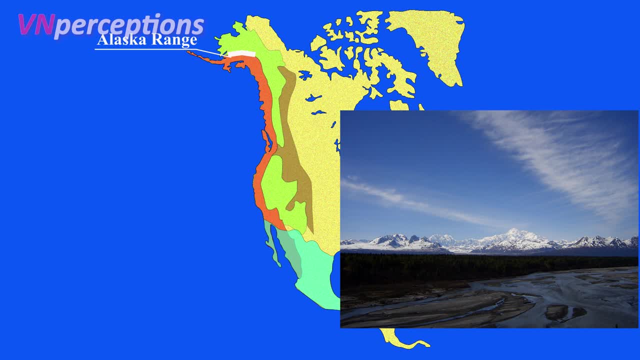 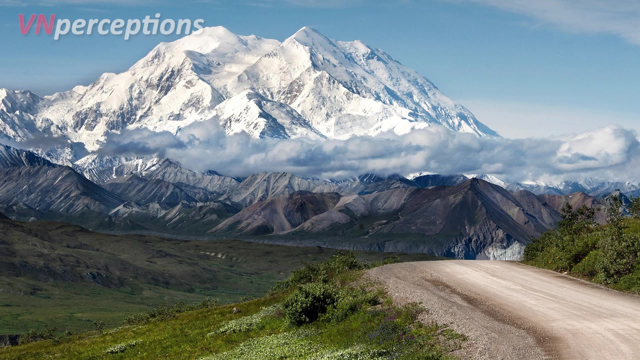 The Alaska Range is a wall of formidable mountains that separates the south central coast from the interior of Alaska. It is best known for its largest mountain, and that is Denali. So Denali is one of the largest mountains on earth and the highest mountain in North America. 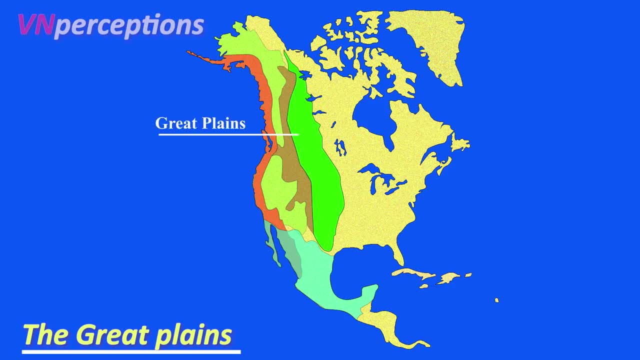 Then we go to the next division, and that is the Great Plains. Well, Great Plains are major physiographic province of North America. The Great Plains lie between the Rio Grande in the south and the delta of the McKenzie River at the Arctic Ocean in the north, and between the interior lowland and the Canadian Shield on the east and the Rocky Mountains on the west. 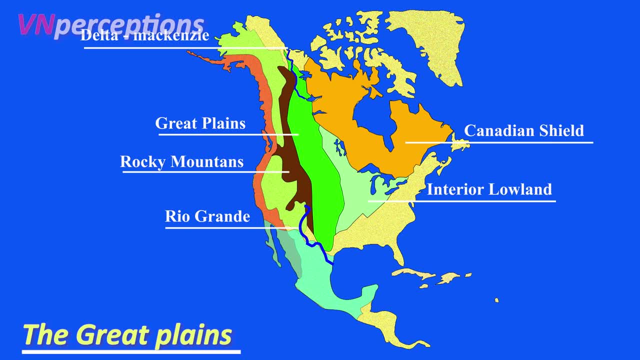 The Great Plains are actually a vast high plateau of semi-arid grasslands. Their altitude at the base of the Rockies in the United States is between 1500 to 1800 m above the sea level. This decreases towards Eastern boundary. The altitudes of the Canadian portion are lower and near the Arctic Ocean the surface is only slightly above sea level. 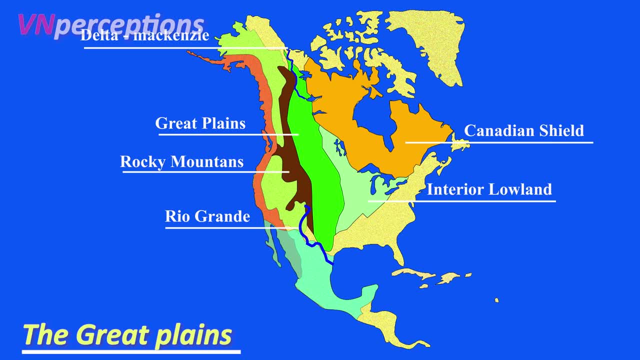 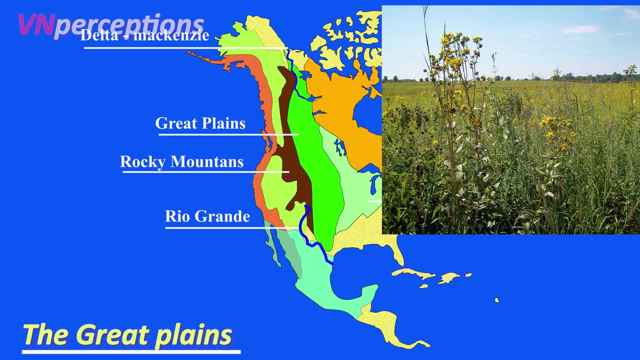 The soil groups of the Great Plains are correlated with rainfall and nightfall. The soil groups of the Great Plains are correlated with rainfall and nightfall. The soil groups of the Great Plains are correlated with rainfall and nightfall, and natural grass cover In the more humid regions with taller, heavier grass cover. 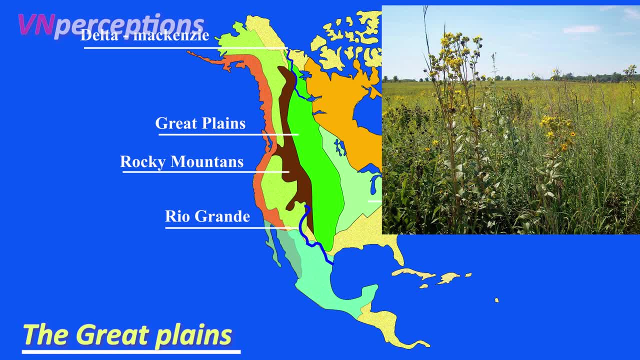 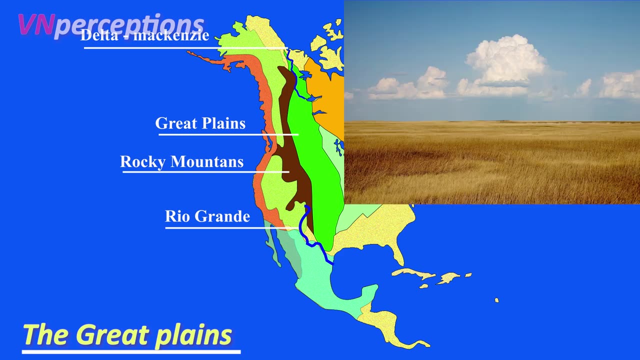 deep black soils with much organic matter is developed. Sections with less moisture have lighter, shallower soils with less organic matter, while in most arid regions the soil are even thinner, lighter in color and less organic in composition. Then we come to the next. 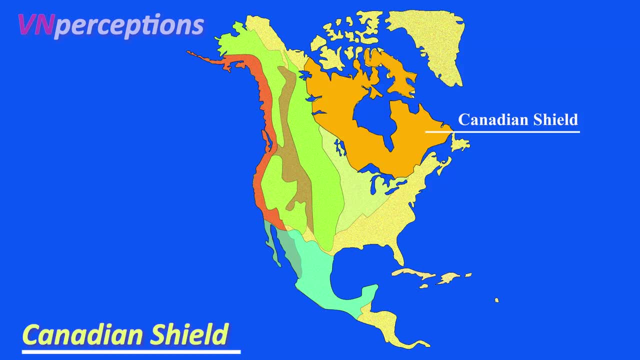 division, and that is the Canadian Shield. The Canadian Shield is the exposed part of the North American Cretan, one section of the earth's floating crust. Well, it is shaped somewhat like a horse hoe or like a shield that ancient warriors used to carry into battle. That's why the word 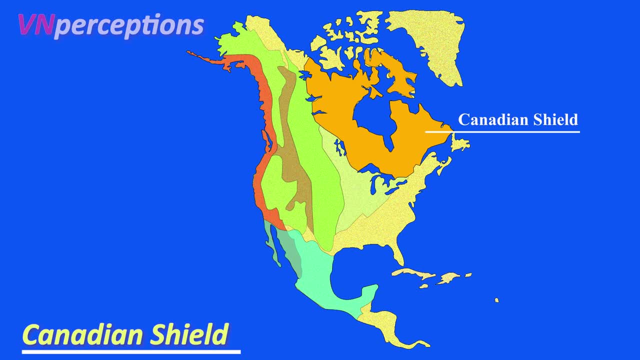 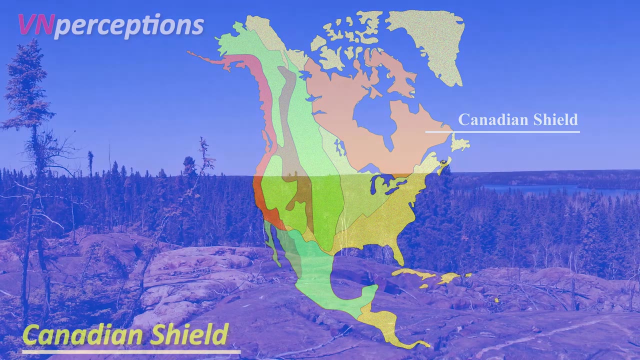 the Canadian Shield. Now this Canadian Shield occupies roughly half of Canada. It occupies the part of North American Cretan, That's on the eastern side of Canada. Unlike the rest of the Cretan, the shield is nearly bare, with only a thin blanket of earth covering its surface. Now, 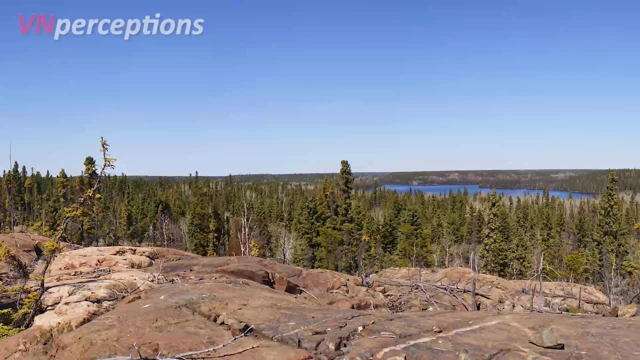 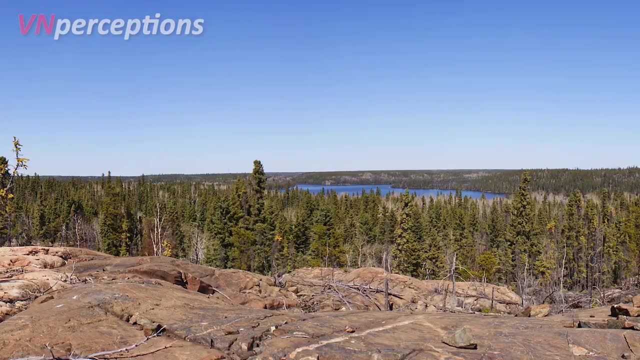 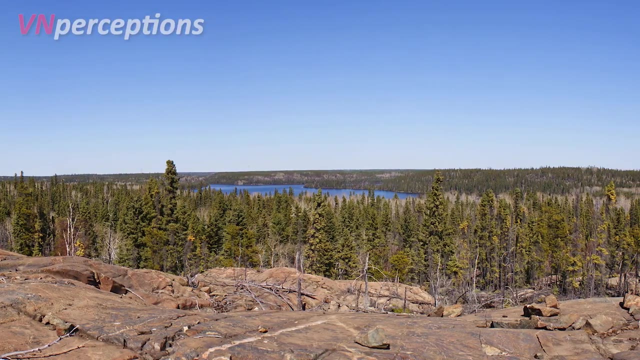 this makes the area much less useful for some activities, such as farming, manufacturing, and more useful for other activities such as mining, logging and hydroelectric power generation. The Canadian Shield is mostly in Canada and from the Labrador Coast on the east the shield covers 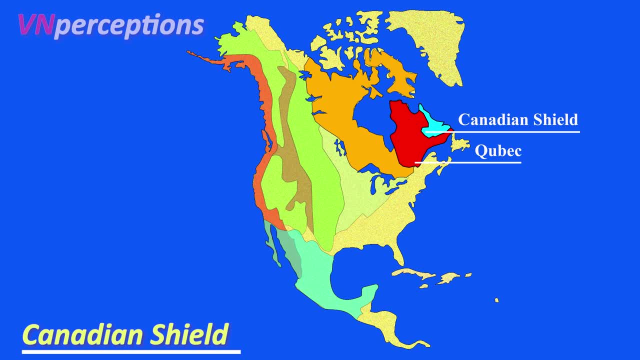 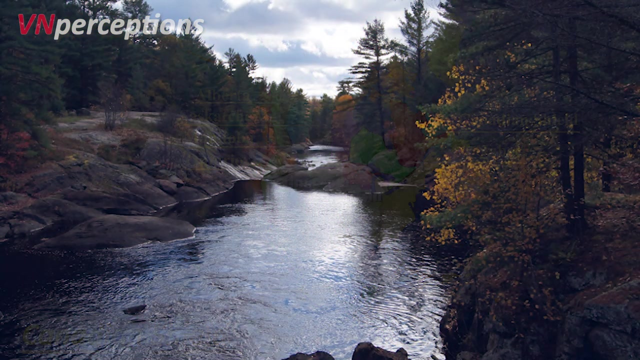 most of Quebec and extends into Ontario, Manitoba, Saskatchewan, Alberta, the Northwest Territories, Nunavut and the Arctic Archipelago. In the United States the same shield, such as Minnesota, New York and Wisconsin. The Canadian Shield's most notable physical features are: 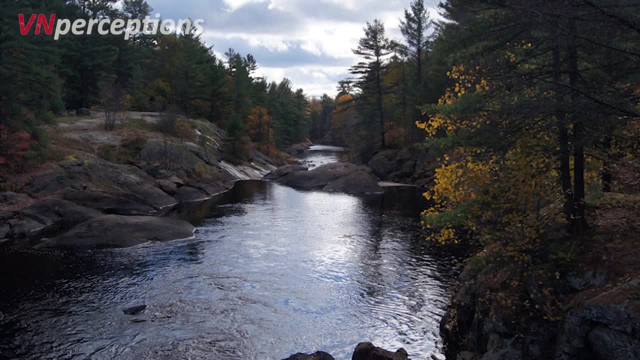 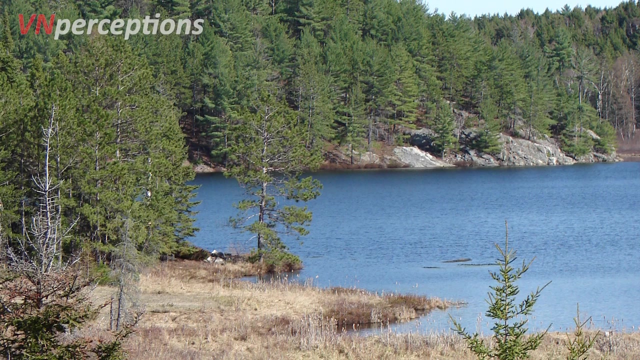 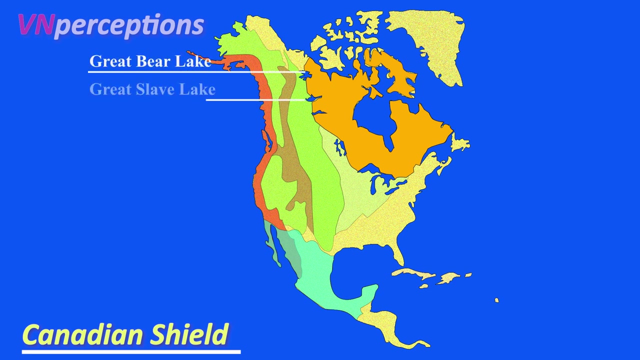 thousands of small lakes, thin layers of soil and rolling hills. Lakes are largely the result of glacial erosion during the last ice age, And the region also borders many of the larger lakes and waterways of Canada. The most significant σουs sand lakes are the lakes of the Great Bear Lake, Great Slave Lake, Lake Athabasca and Lake Winnipeg. 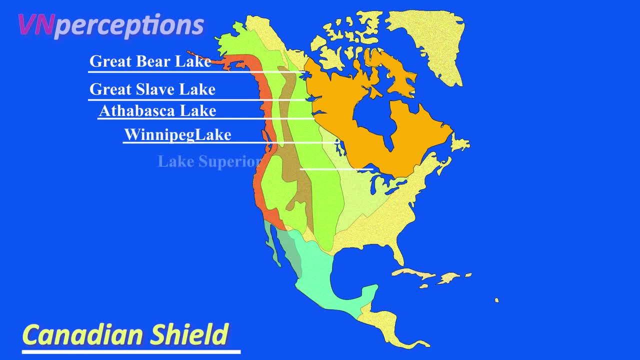 Nothong shores of the Lake of Woods, Lake Superior, Lake Huron and the North Shore of the St Lawrence River also have lake sources. The Other lakes are Lake Michigan, Lake Eric and Lakegeb- describing for you the Jeremy River- The Loufer and�idonakan lakes in the Lake of Woodland. 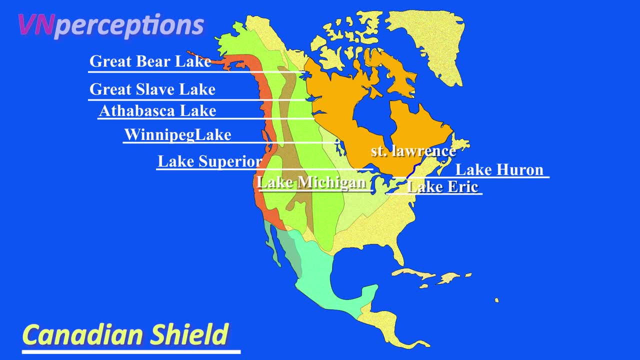 Now they most commonly seating at lower theIPCC, Hillwall, Then in the St Raphael River, Lakeplacid River, Camberley, where it is privately Vine Butler, and imbalance Lake Ontario Coming to next, and that is the Varied Eastern Region. Well, the Varied Eastern 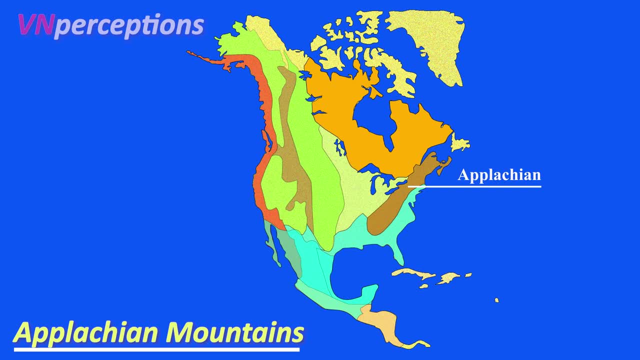 Region includes the Appalachian Mountains and the Atlantic Coastal Plains. The Appalachian Mountains are called the Great Highland System of North America, the eastern counterpart of the Rocky Mountains. They are the oldest mountains on the earth and they lie partly in Canada but mostly in United States. The whole system may be divided into three great sections, and they are: 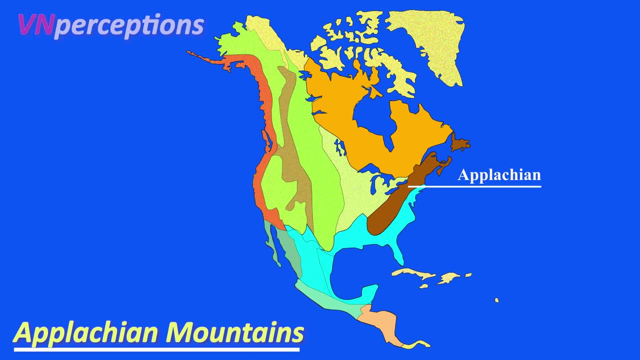 the northern. The northern section runs from the Canadian province of Newfoundland and Labrador to the Hudson River. The central part goes from the Hudson Valley to the New River, that is, the Great Convalescent. The southern section runs from the New River onwards. Next division is the Coastal Plains. 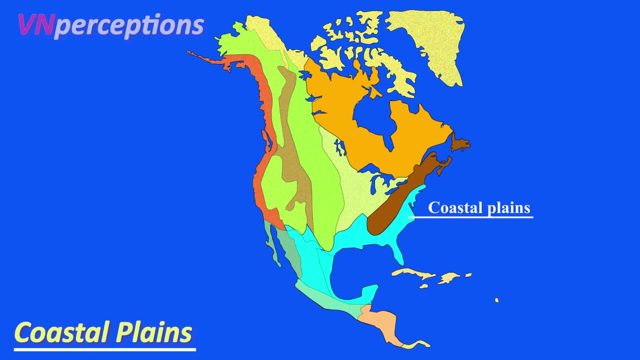 Well, the Coastal Plains is one of the largest province in the eastern North America. The Coastal Plains begins in Mexico and the Yucatan Peninsula, extends through the Gulf Coast and Atlantic seaboard states and ends at the Cape Cod, Massachusetts. Now, these are. 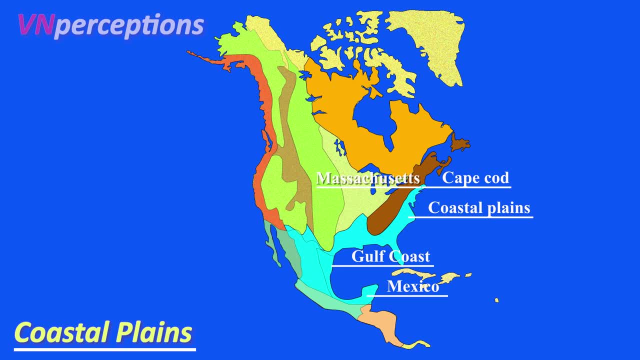 a large part of the Coastal Plains. The Coastal Plains is one of the largest province in the United States. It is a lowland, mostly flat area that stretches 3200 kilometers from Cape Cod, then along the Atlantic coast to west into Mexico. The average elevation is less than 200 meters. 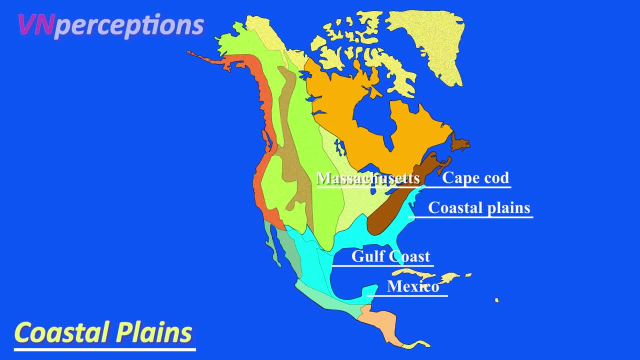 above sea level. More than half of the Coastal Plains is less than 30 meters above sea level and it contains much of wetlands, mostly swarms and marshes. Both are sources of shellfish and many other aquatic life forms. The Mississippi Delta is where the Mississippi River empties into. 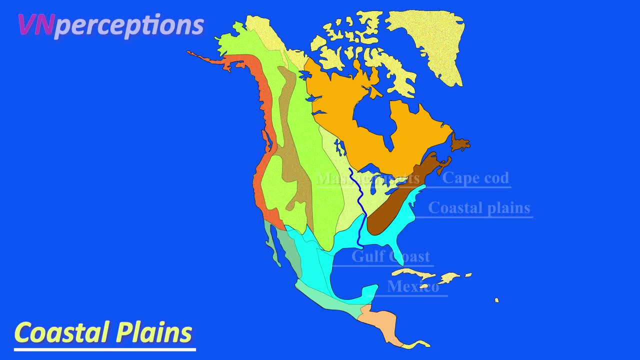 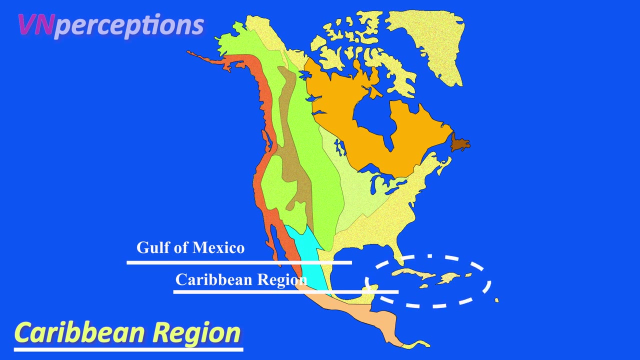 the Gulf of Mexico, creating large areas of fertile land used for agriculture. Finally, we come to the Caribbean region. The region is southeast of the Gulf of Mexico and the North American mainland, east of Central America and north of South America. It is situated largely on the Caribbean coast.